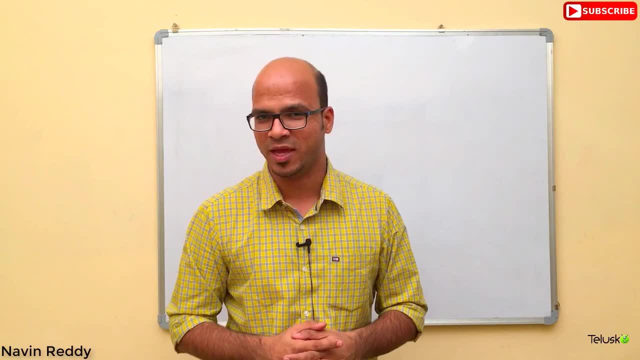 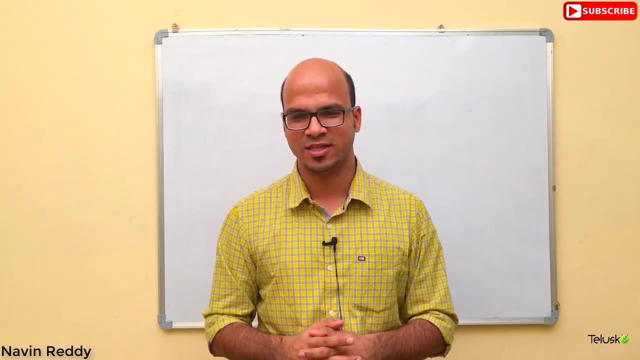 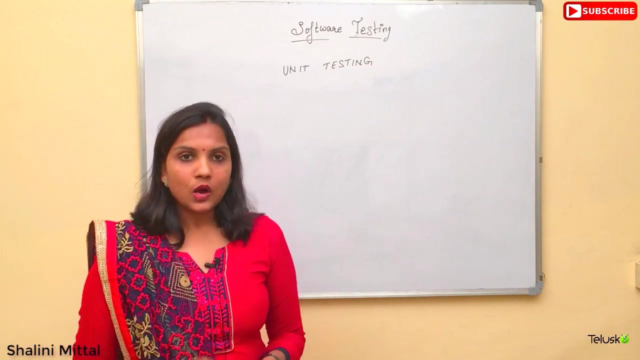 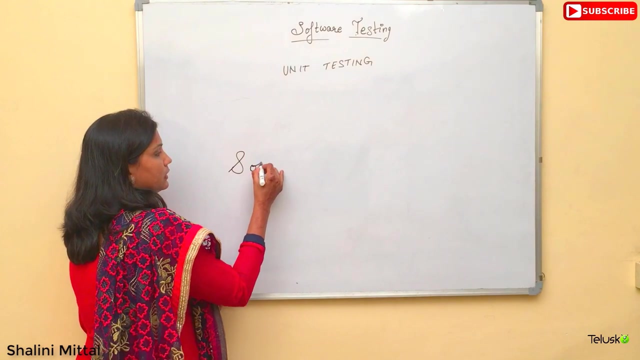 So for testing, for development, she has done the training for all these domains, And so let me introduce Shalini Mittal, and she'll be talking about what is unit testing and what is software testing in this video. Hello, friends, and this is Shalini Mittal, and I welcome you all on this small demo on unit testing. Now, the topic for today will be unit testing, which comes under a part of software testing. Now, software, we all know that's a system that we create for make our jobs easier. 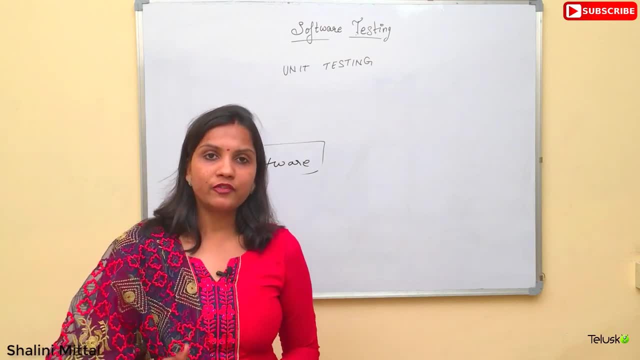 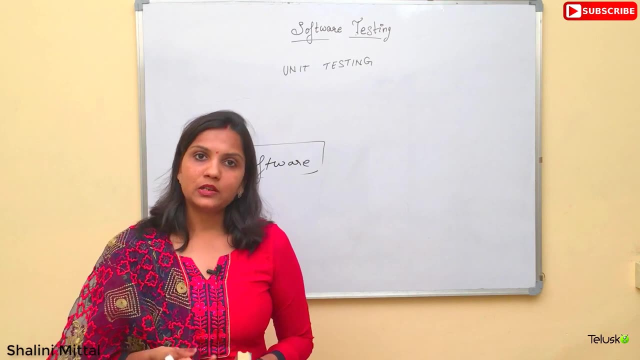 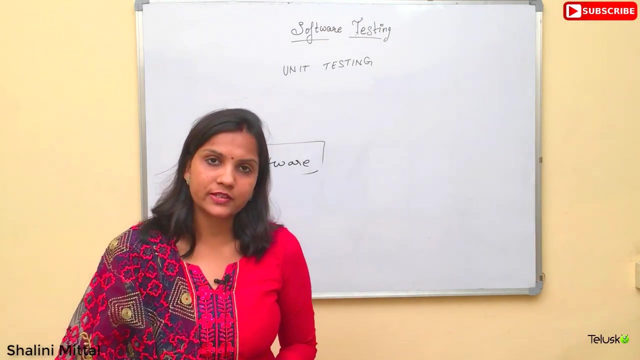 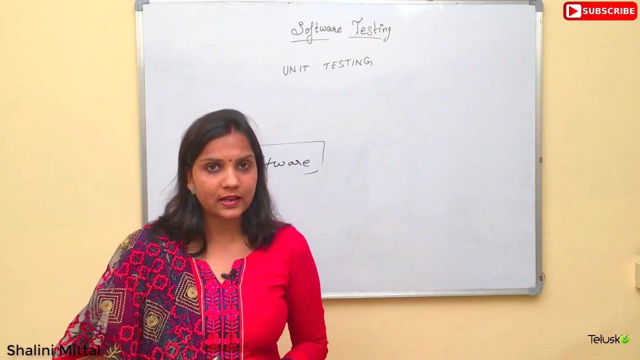 So software creation, or when I say software, when we get the requirements, So basically software in a whole- starts from the moment you get the requirements from the client. You assess the requirements, you analyze them and then you create the designs for them. We have the design structure, Then you go ahead for the implementations of the same Of course. then there are life cycles, like you go for testing, and then the quality assurance, the user acceptance testing, You go and deploy on the client side And then later on, when everything gets approved, is when you actually deploy the software or the application. 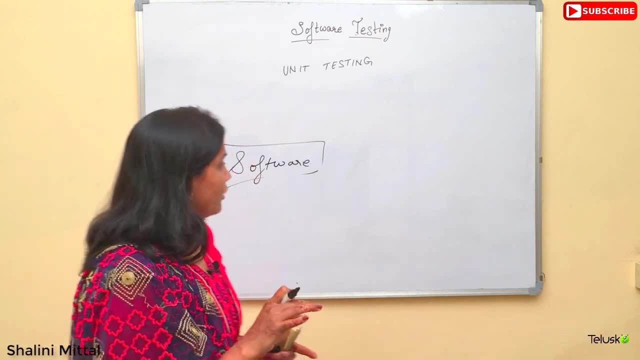 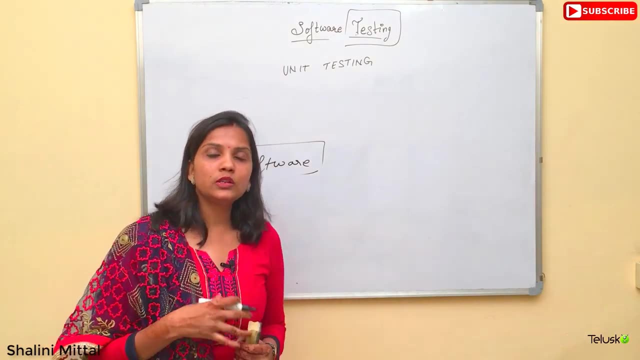 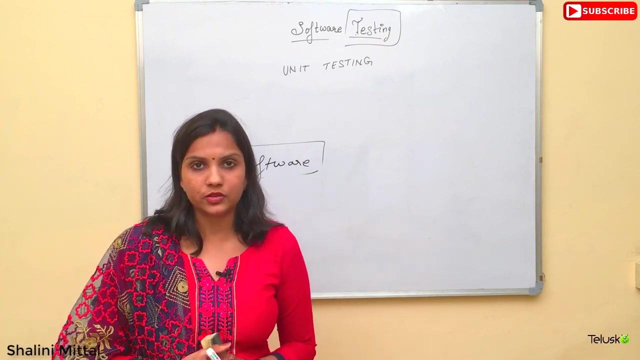 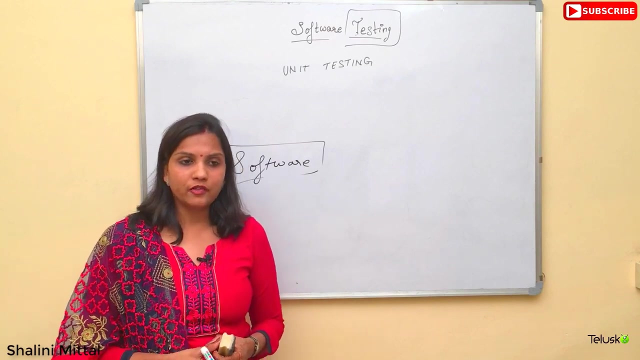 Created by you on the client side. Software testing starts from the moment you start with getting the business requirements. So it's suggested that earlier you do the testing, Better it is for you to get less bugs, less errors and create a more error free applications. Now, what is testing and why it is needed? I guess in day to day life, suppose when I'm going for any shopping, right If I'm just buying apples, Every time I do test each and every apple and I do touch them. 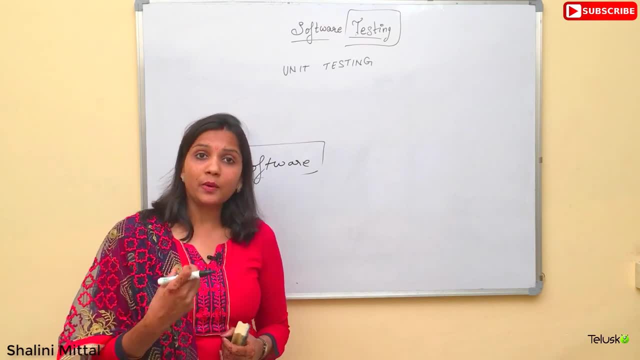 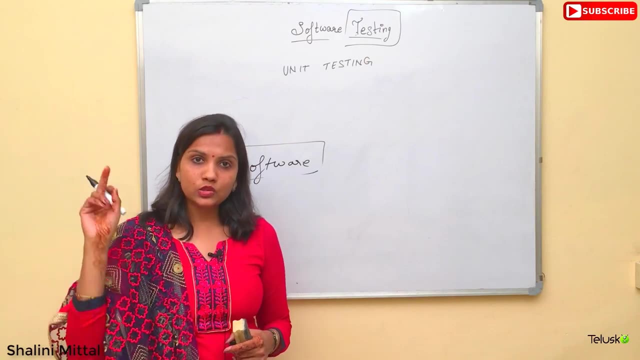 touch it, maybe smell it or maybe. I ask lots of questions even before buying anything. why was I paying money for that? we do testing at each and every phase of our life. you get up in the morning, you switch on the light. if it's working or not, I go in the kitchen. 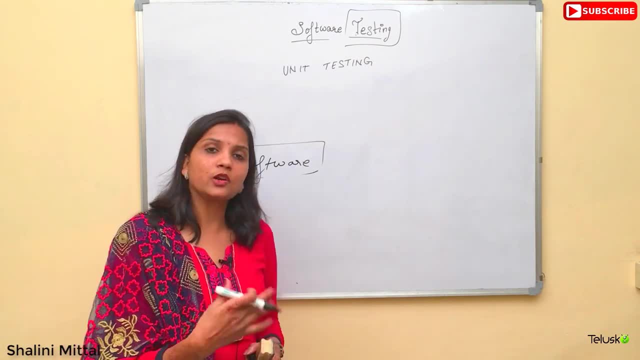 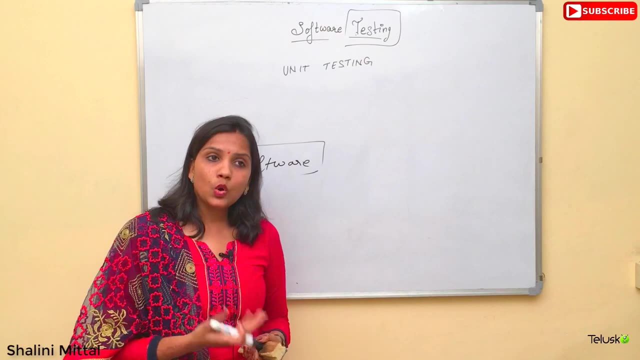 in the kitchen, when I am working. I do testing at every part of my life, at every part of the stage. it's just, it's so natural to us that we don't realize it's a part of our life that we are doing testing at all the times. we go and inquire for any classes. now, for 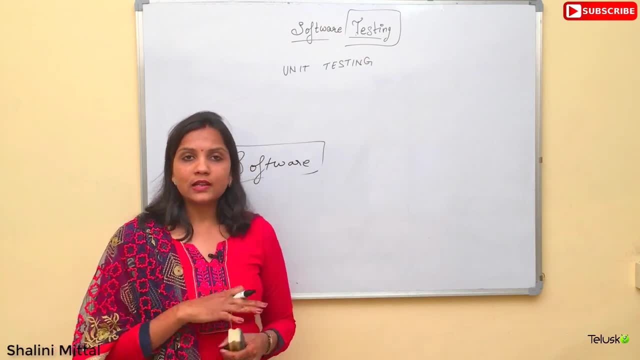 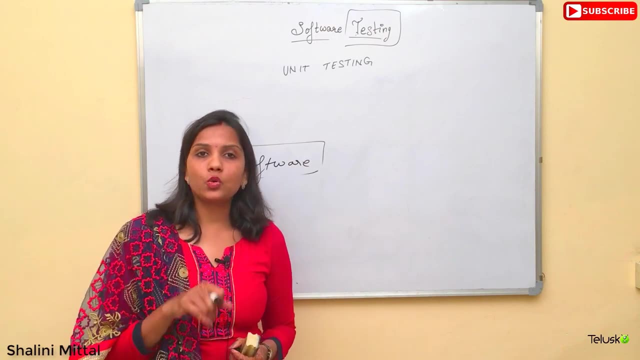 example, you want to come for this class as well. it's not that you inquire at one class and that's it. you join them. you inquire at many places. now, what's the reason behind that? of course it's you want to get better quality for the money that you are paying. 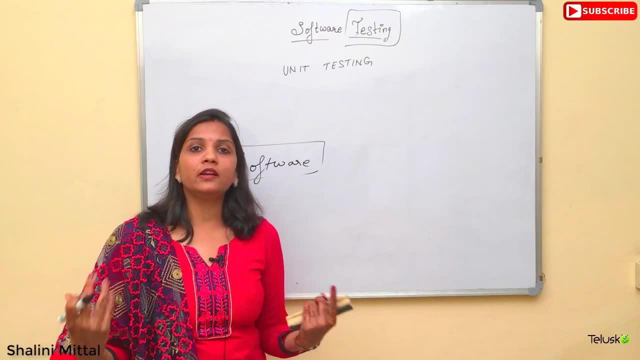 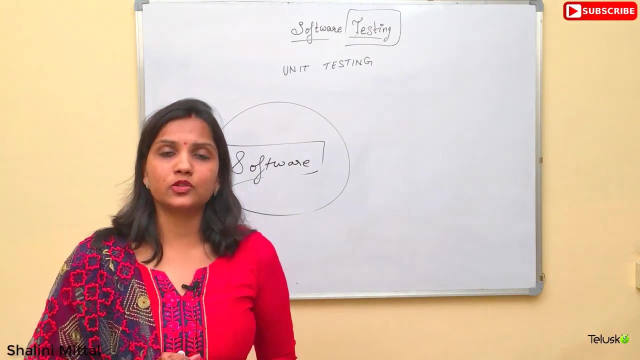 so testing at every phase in our real life. we have it in and around us. so then, why not include that testing in our software development life cycle? of course, when I talk about the software development life cycle, or the phases of software development, we have it starts. 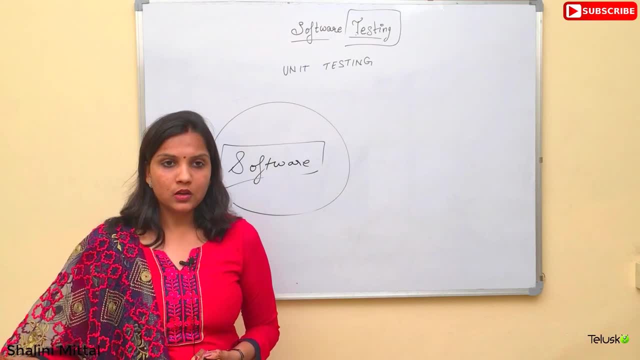 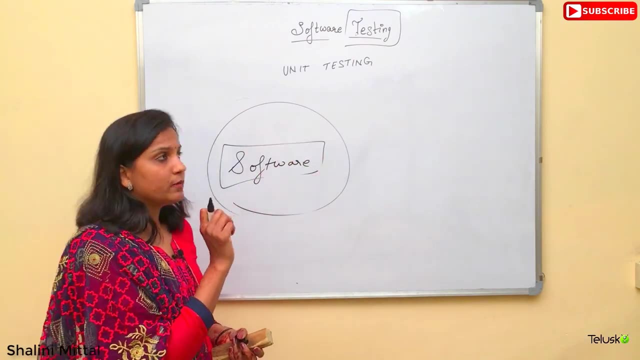 with the requirements gathering to the design, to the implementation, to the testing part, to quality assurance, and go on and further today's topic. I won't be focusing on the whole life cycle, but I will be focusing on one part of the software. 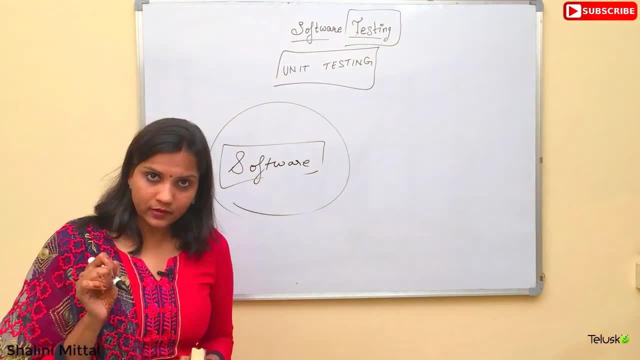 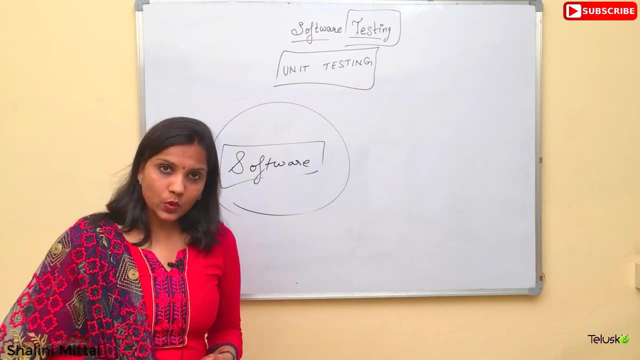 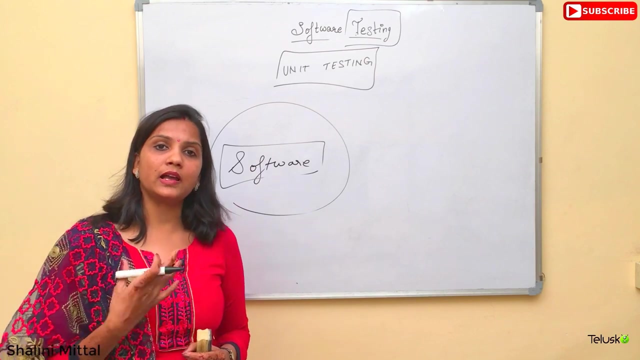 testing, that is, unit testing, now by unit. that term comes along with testing now as discussed, testing we know that we require so that we get better quality. like we know in advance that whatever we are delivering it is as far as with power to the client's. requirements and less error process. So unit testing unit implies that the smallest unit in your particular modules that you can test, a unit testing. if you compare in terms of java, the smallest unit in a java program is nothing but a class, and classes has method. so you basically try to test the functionality. 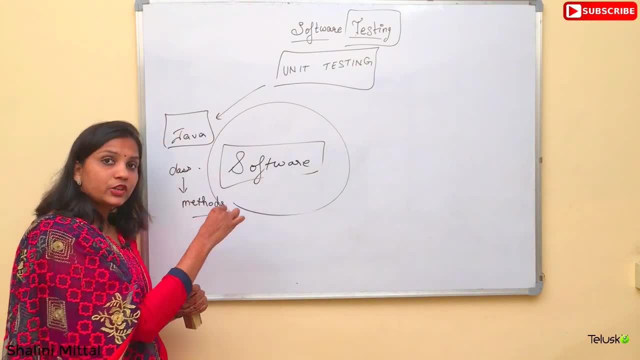 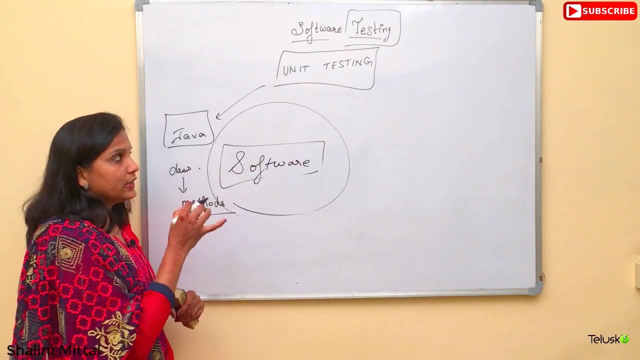 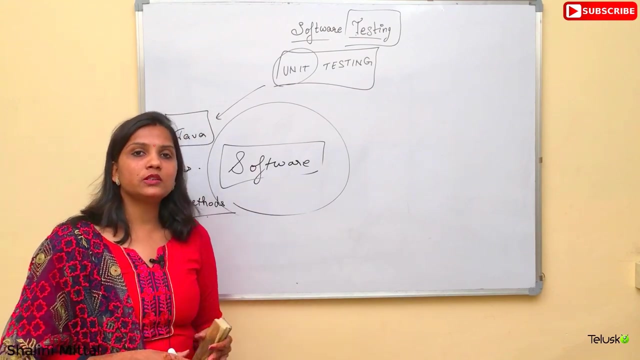 of how the classes or the methods that you have designed. they are going to work independently, irrespective of in and around situations. So that's it. So that is what it means by unit testing. that is, we are going to test each and every small module of our application, and smallest module in java application is nothing but. 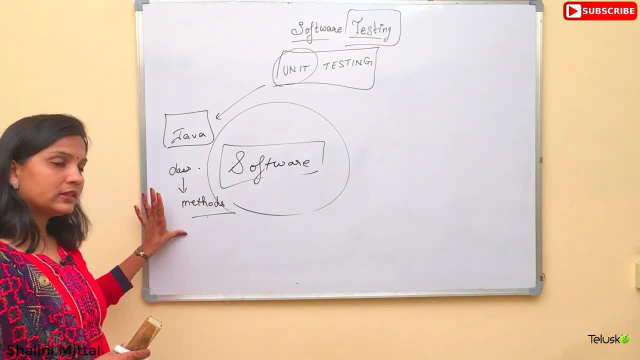 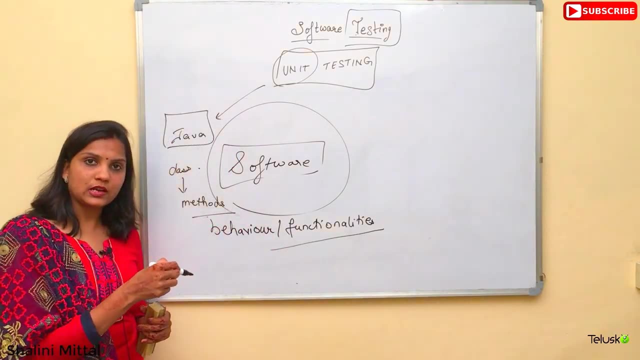 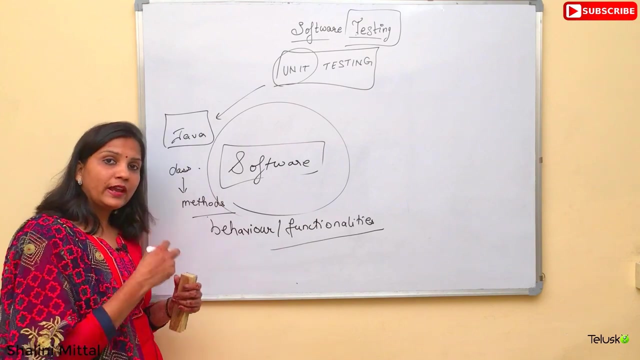 a class. class comprises of methods, and methods has what behaviour? or I can say it consists of functionality. Each individual piece of our classes. we would want to go for testing, setting the expectations, what exactly we expect, and then running it and testing it and seeing it, whether, whatever. 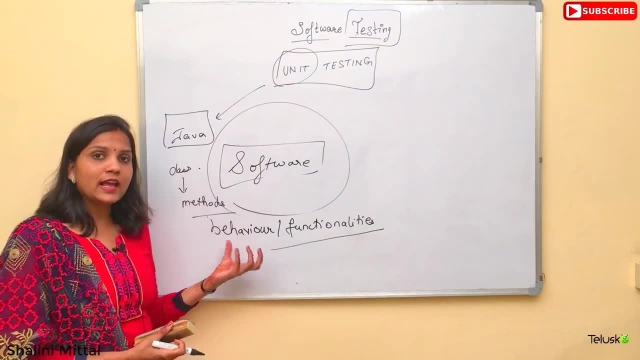 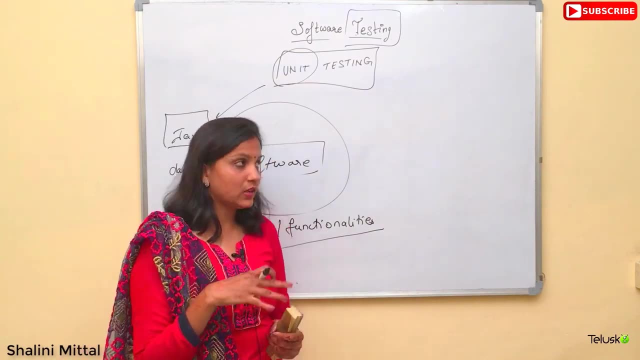 expectation. expectation is there, we are going to test it. So what are the expectations we had from our modules? is it actually performing the way that we expected to, right? So we are going to test the functionalities. Now, before I dwell into the J unit testing or the unit testing, we just have a quick. over look as to all the available life cycle phases in software testing. We have unit testing, we have integration testing, we have system testing, we have user acceptance testing and when at the last, we have the release. So we have the integration testing, we have system testing, we have user acceptance testing. and when, at the last, we have the release. So unit testing is the part which is done by the developer. So developers are responsible for providing the unit testing within their applications: Integration testing, system testing. then you have the various testers available who? 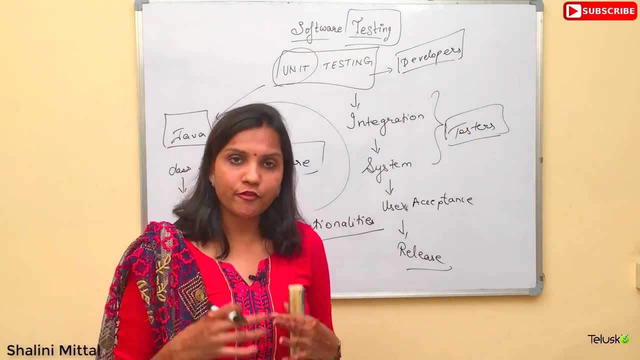 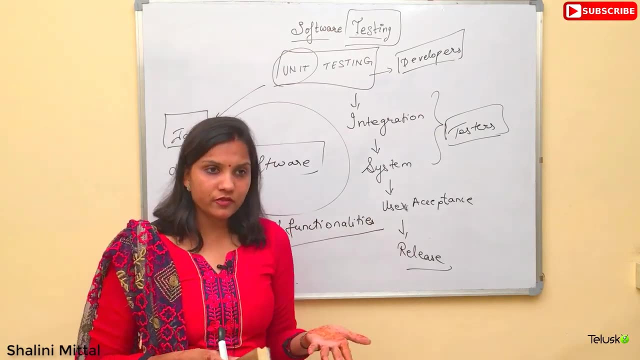 are responsible, then, to integrate all the modules, first one by one, test them and then the whole system integrated as a whole. Now, when I talk about system, system may imply you have servers, you have databases, you have the browsers, you have the machines, you have the operating systems, you have the 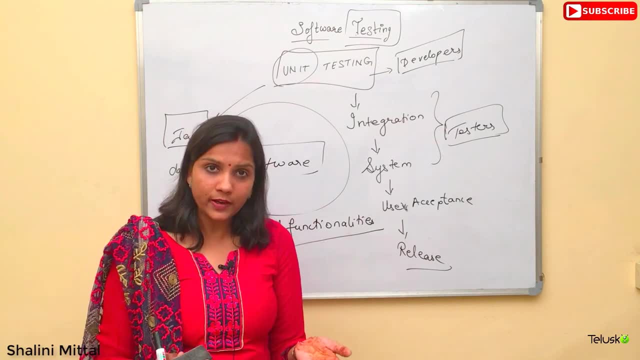 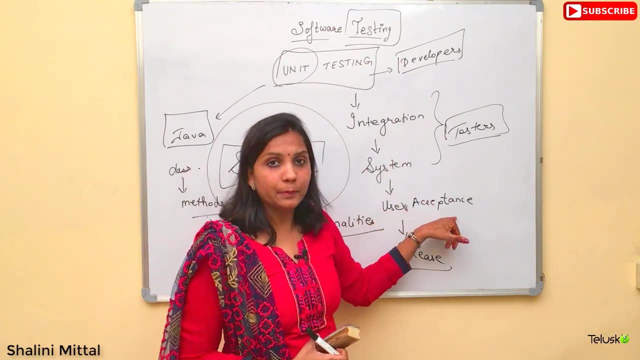 software itself. System implies testing each and everything that's included into your applications We go about. once the testing is done from our side, then we go with the user acceptance testing. It is nothing but the user, that is the client. he basically then test it. 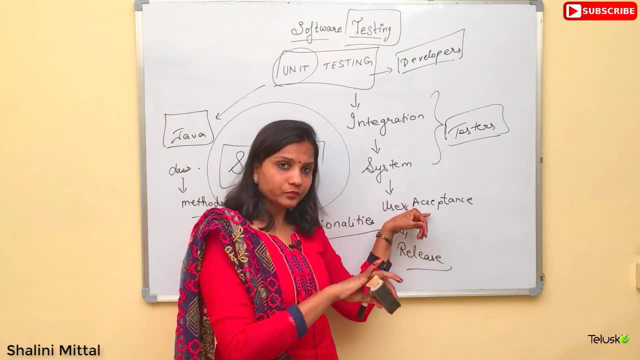 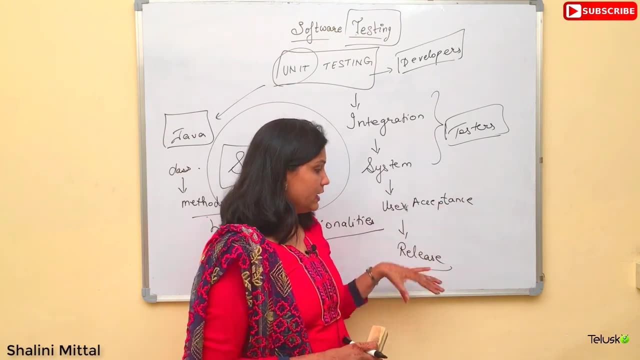 Now this testing can be done at the client side or it can be done at the service provider side. Once the user acceptance testing is done and the application is with the power of the requirements of the client, then it goes for the release testing- Again release. you have two versions. 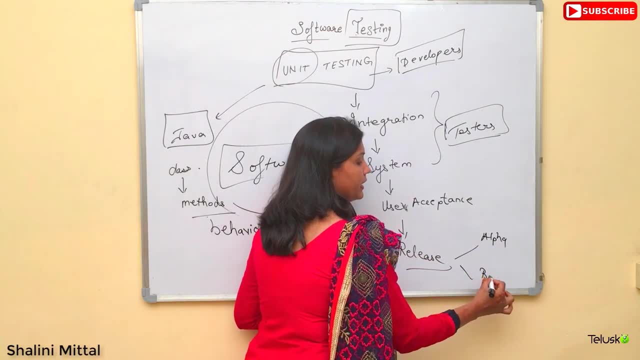 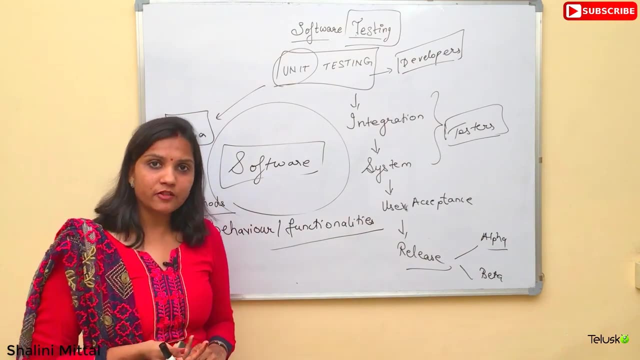 You have the other version, You have the application, You have the alpha and you have the beta version. So alpha version is still again in the testing phase, and then you have the beta versions. Again, there are few testing strategies available, like we have testing strategies. 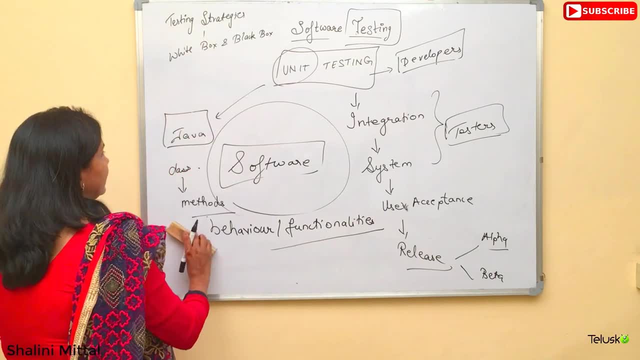 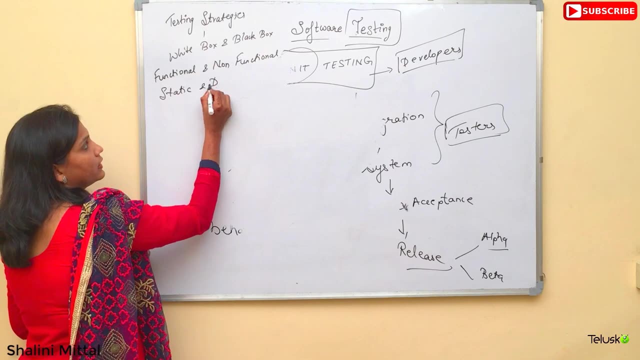 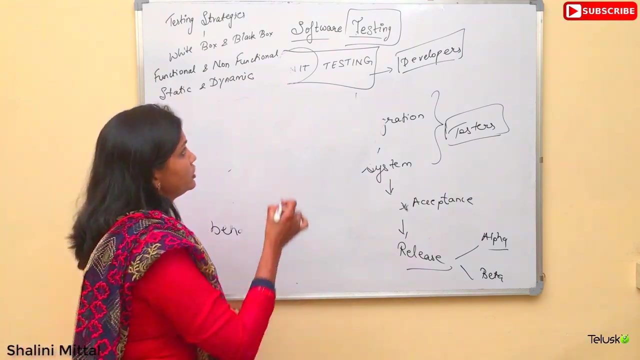 They are white box and black box testing. Then next we have functional and non-functional testing, We have static and dynamic testing. Okay, So we have all these kinds of testing strategies available. Okay, So what is the testing strategy? The testing strategy is a kind of white box testing, out of which the unit testing is a 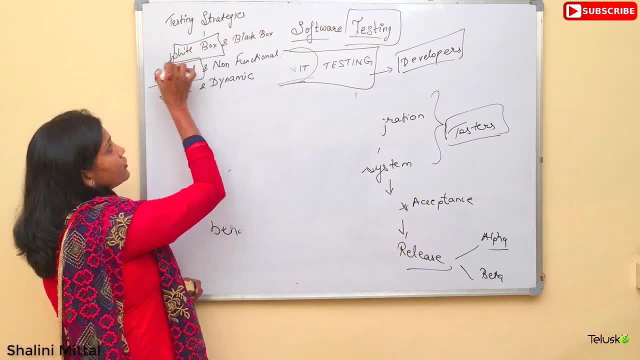 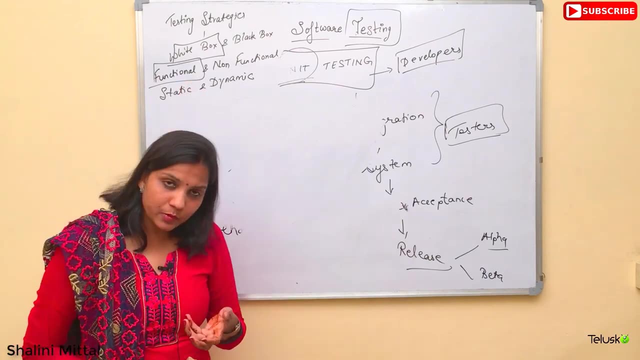 kind of white box testing, wherein we are going to test for the functionalities in our application and this testing can be static or can be dynamic. Now, when I talk about white box testing, it implies that I, as a developer, knows in and out of the code. 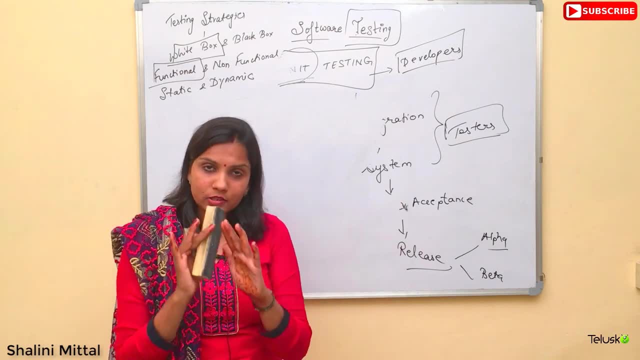 I can actually view. I know every line written because it's all white. It's open to me When I talk about black box testing that's done by the testers, wherein they don't know about the coding that's being done behind the scenes. 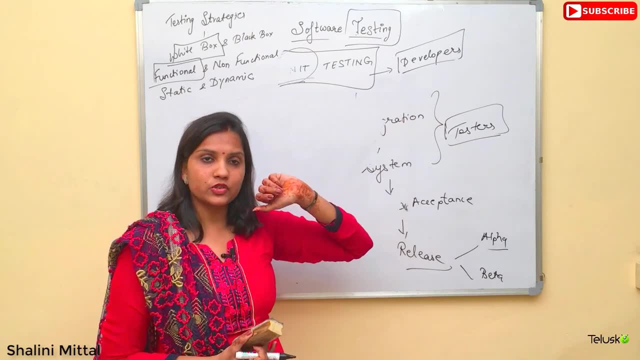 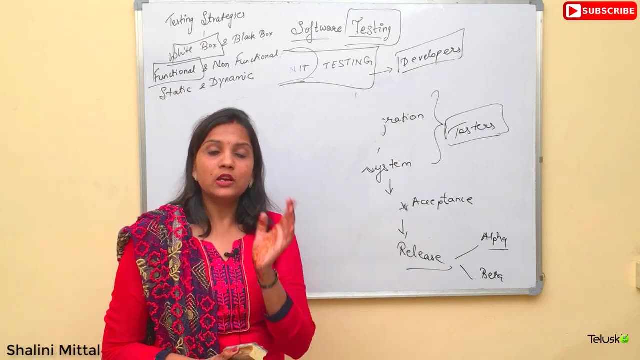 They just check for the functionality, For example a login application, so they might be testing whether the login application, when I log in, does it redirects to a login page or to an error page. does the second page comes up or not? or when I click on a button and login credentials are wrong in 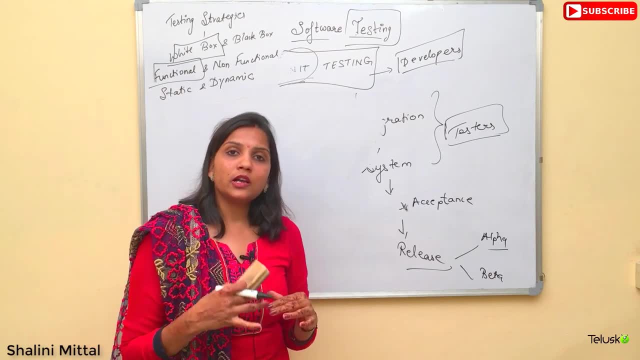 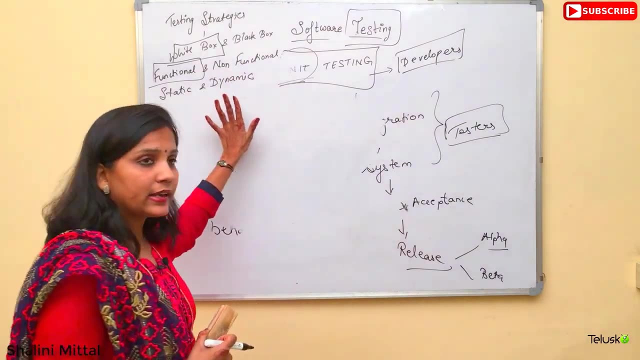 that case, does it display the error messages properly or not? right, This is all done by the testers, which comes under the black box testing. We have functional and non-functional requirements in our applications. We also have static and dynamic testing, wherein static testing is: I'm writing my code and 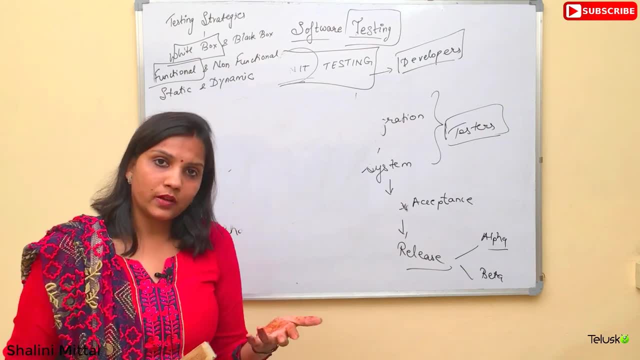 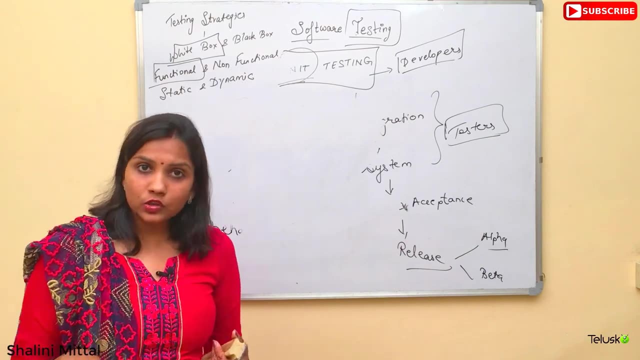 I want it to be get reviewed by my peers, Okay, Or by my managers, or my managers or anyone, So they are not actually executing the code. The only thing is they are basically reviewing it. So it can be documents reviews, walkthrough reviews. 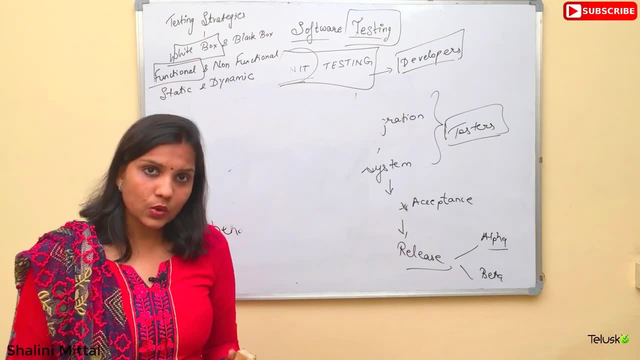 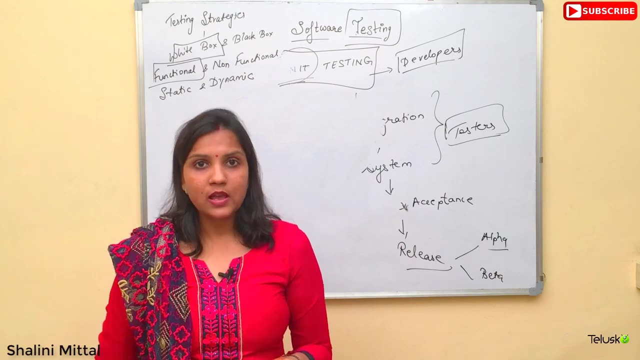 It can be done without executing the code. So if you are not executing the code, getting it reviewed by your peers, it is called a static testing. Dynamic testing is when you actually start the execution of your programs and you are actually testing it. what's the output of your applications? 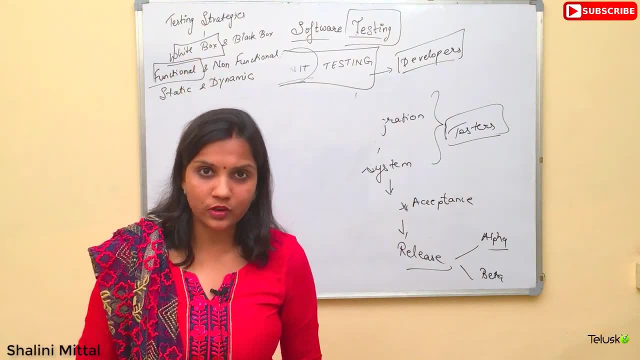 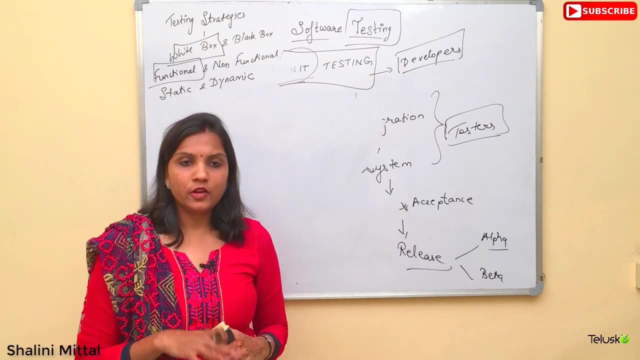 So we have few testing strategies and, of course, nothing goes if you don't have some principles, rules to follow. should we check for all the possibilities, even for the negative values? yes, why not? right, when you buy a car, the car before being on roads it's being tested and driven through all kinds of 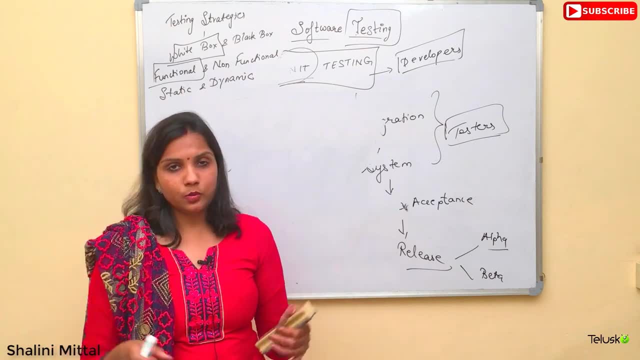 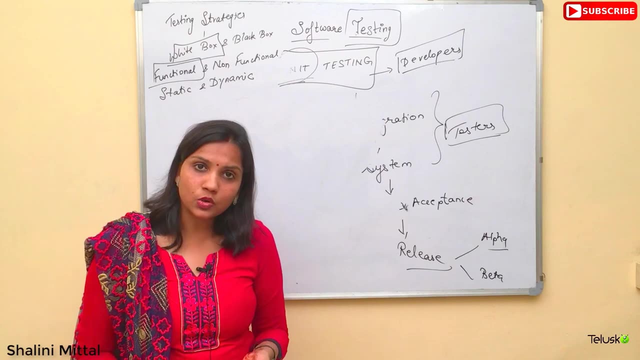 conditions. it's not tested only for the ideal conditions. especially when i go to buy a car, i will not test a car on the smooth road. i'll definitely take the car onto the road where there will be bumpers or there will be potholes or their roads should be curvy, and test it so that. 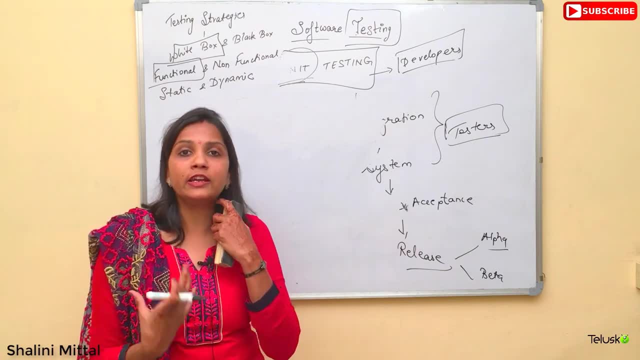 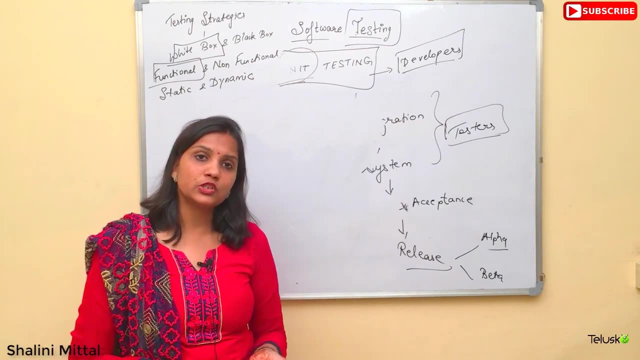 while i'm buying a car, i know that it will. it will run on indian roads, specifically on the indian roads, right? so when in real life we go on about all these testing principles, why not apply all these rules into our software applications as well? so always remember: you need to test for all. 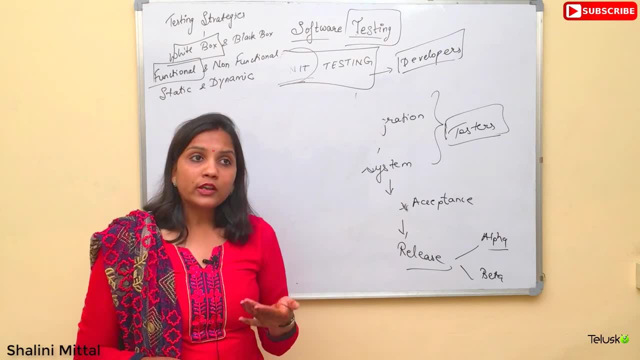 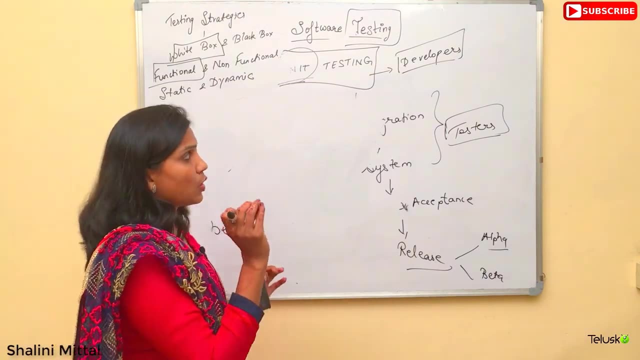 kinds of scenarios do not work for only ideal conditions. whatever possible values you think are impossible should still you should- test for all the impossible values as well. so this is all about a small overview on to what is software testing now. the main topic for today is unit. 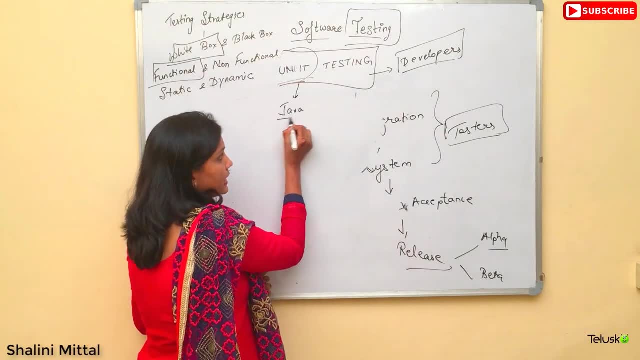 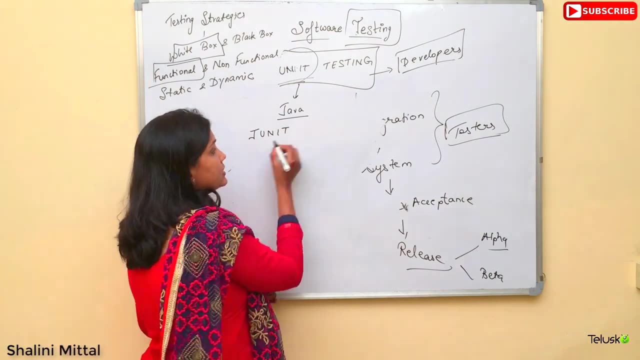 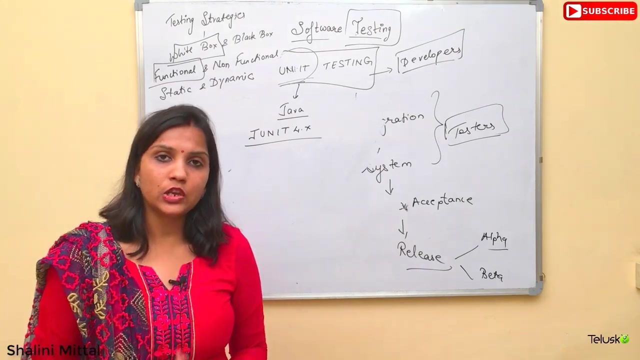 testing, now unit testing with respect to java, is done by using a library called as j unit. now, the version that you will be learning today, that is j unit 4, so it's j unit 4.x. so we had j unit 3, which had few drawbacks. so we have j unit 4, which comes in with rich features of code java wherein it. 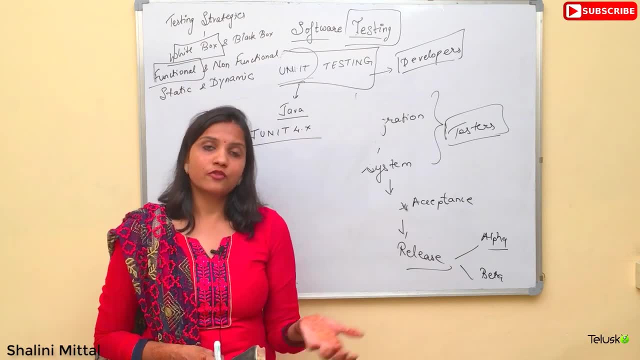 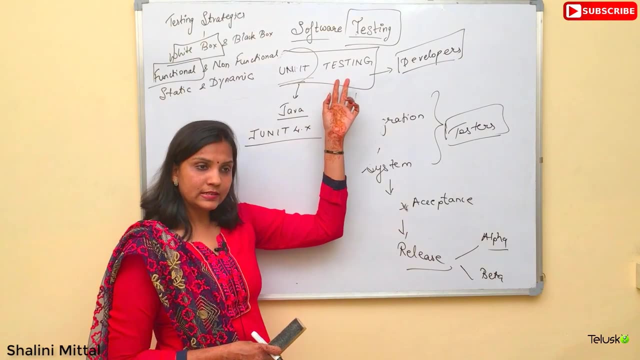 supports annotations, then it gives you the flexibilities of adding the libraries and getting your work done in a faster way. so the topic, the library that we are going to use so for unit testing, is nothing but j unit 4. is installation tough for j unit 4? not at all. you.